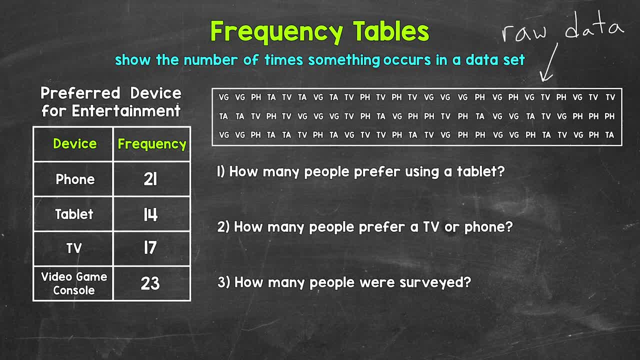 this is pretty difficult to interpret and understand, as is A frequency table will help us organize everything, And our table is right here to the left. So, as far as this table goes, the left column shows the devices and then the right column shows the frequency, The number of times each device shows up within the data. Now, as far as 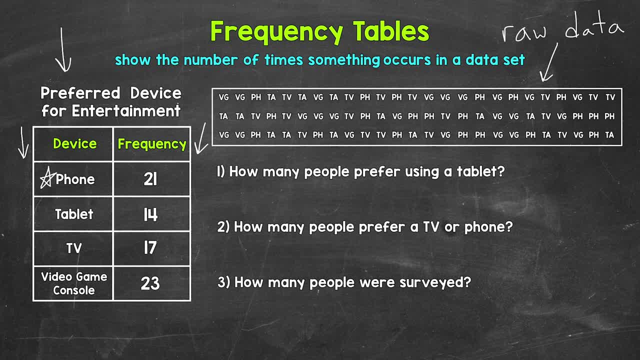 reading this table, we can see that for a phone, we have 21 people that prefer that device. For a tablet, we have 14 people, For a TV, we have 17 people, And then, lastly, for a video game. 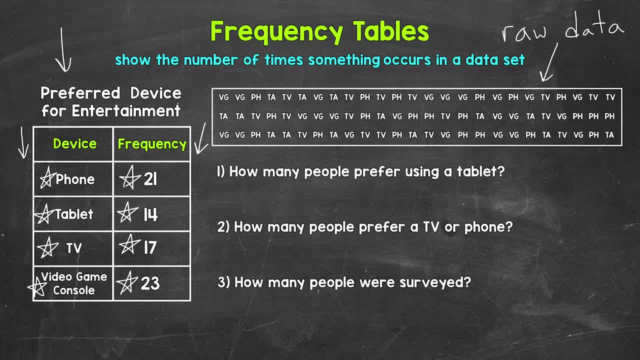 council, we have 23 people. You can see that this frequency table really helps organize and present the data in a more meaningful way. Now let's answer some questions, Starting with number one, where we have how many people prefer using a tablet. 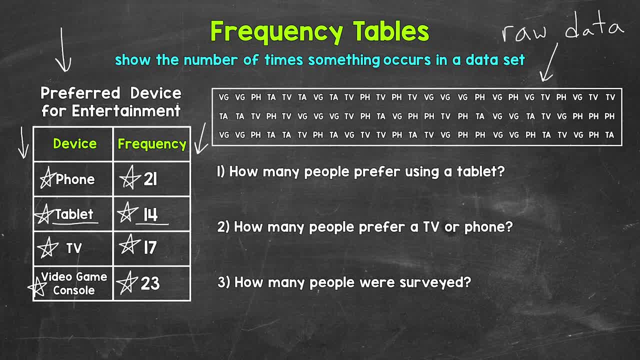 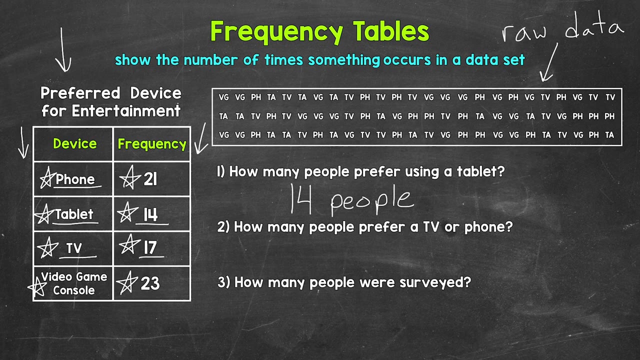 Well, tablet is right here and we have 14 people, So 14 people prefer using a tablet. Let's move onto number two, Where we have how many people prefer a TV or phone. So we need to look at TV and phone. So we have 17 for TV and 21. 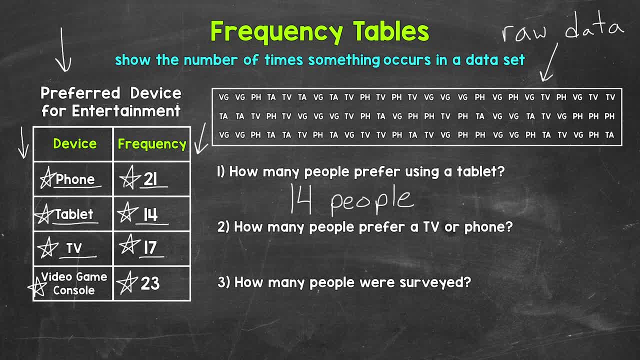 for phone. So people plus 21 people gives us 38 people. So 38 people prefer a TV or a phone. And then, lastly, for number three, we have how many people were surveyed. So for this one, what we need to do. 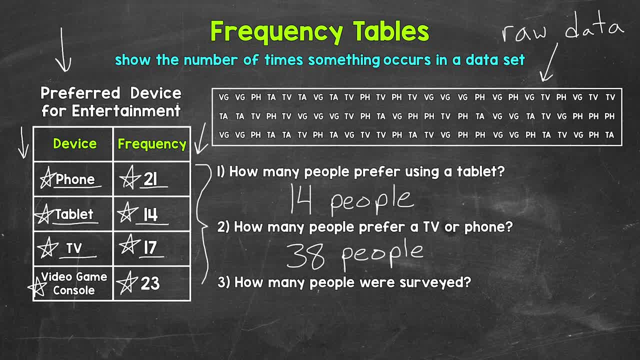 we need to add all of the numbers in the frequency column. So 21 people plus 14 people plus 17 people plus 23 people. 21 plus 14 is 35.. 35 plus 17 is 52. And then 52 plus 23 gives us a total. 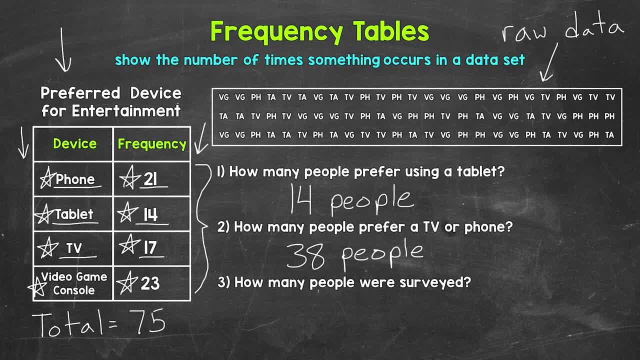 of 75.. So how many people were surveyed? 75 people. So there you have it. There are the basics of reading and understanding a frequency table. I'll see you in the next video. I hope that helped. Thanks so much for watching. Until next time, peace.